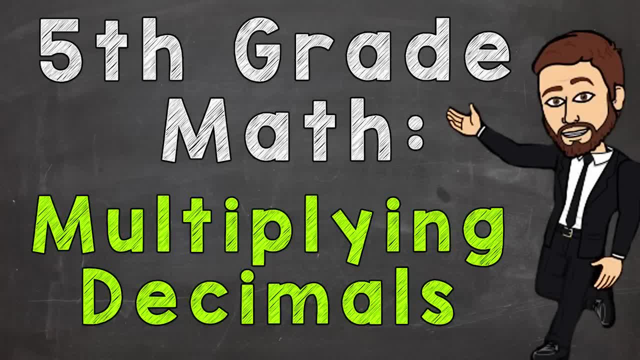 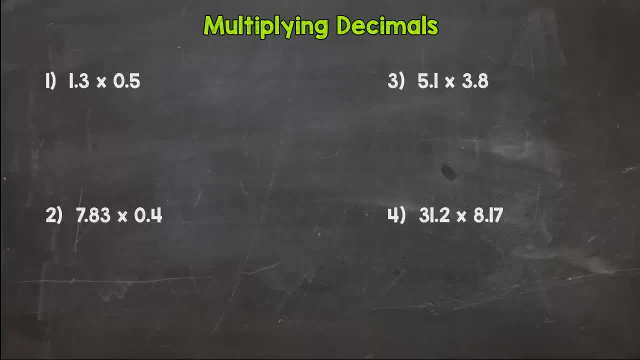 Welcome to 5th grade math with Mr J. So in this video we are obviously going to be multiplying decimals. Now, multiplying decimals is very similar to multiplying whole numbers. It's really the same exact process, except for the end, when we have our answer, we need to make sure we place the decimal in the correct place. So if you have the process of multiplying whole numbers down, you will be in good shape to start off. If you need a little. 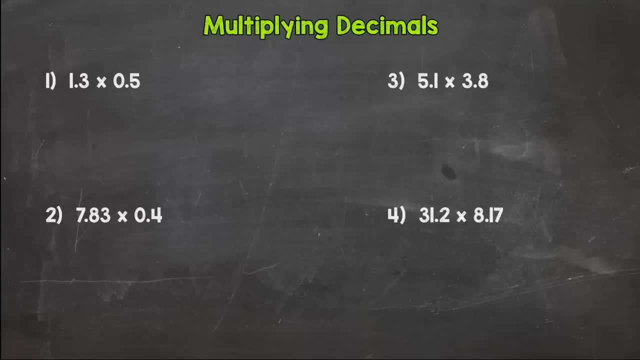 review on multiplying whole decimals. I drop the link to my instructional video below and then you can come back to the decimal ones. So let's hop into number one and, as you can see, we have four problems here. We are going to go through these four problems together. I suggest writing them out with me on paper and then we'll try a mastery check where you'll try some on your own to see if you have it down. So our first rule for multiplying decimals is we need to rewrite the problem vertically. So we have 1 and 3 tens. 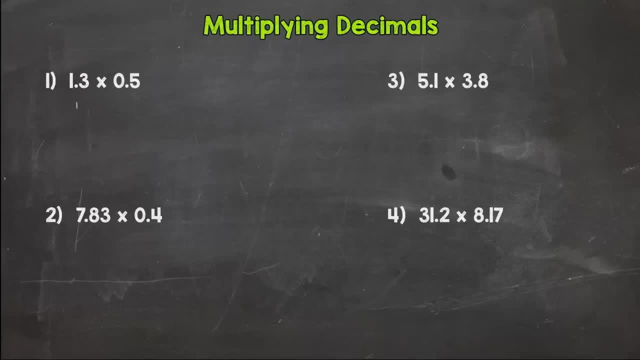 times 5 tens. So the first thing I like to do is take the decimal out when we write our problem. So I would just write 13 times 5.. You don't need to line up your decimal when you multiply decimals, like when you have to in adding and subtracting decimals. This is a different process. So take the decimal out and 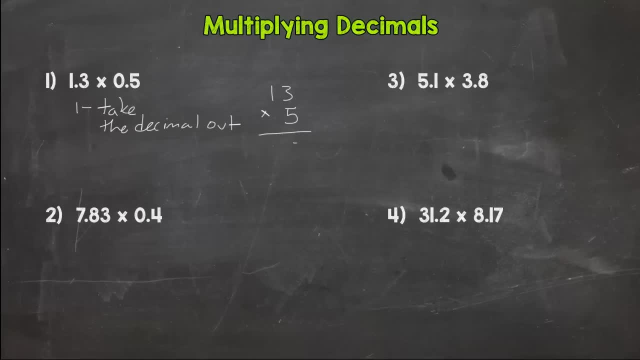 do 13 times 5.. 5 times 3 is 15.. 5 times 1 is 5 plus 1 is 6 and we get 65. Now our answer is not 65. Take a look at our original problem. 65 doesn't make sense for that problem. So what we do in order to place the decimal, we count or see how many digits are to the right of a decimal, And we have this 5 here and we have this 3.. 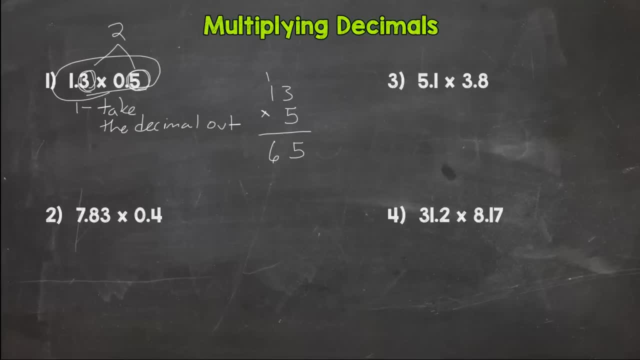 so we have two digits behind or to the right of decimals. so that means your answer will have two digits or numbers behind the decimal. so we bring our decimal in twice one, two, so our answer would be 65 hundredths. okay, pretty easy. so first step, take the decimal out, go through your multiplication. 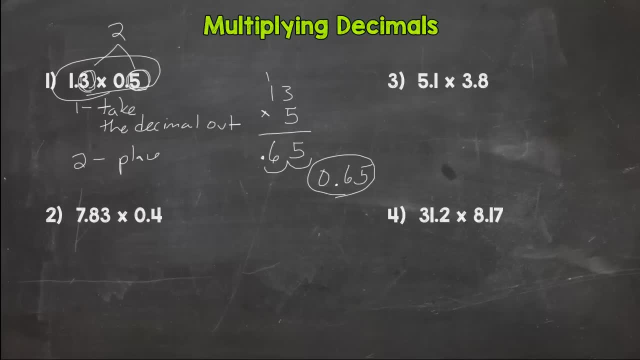 process. second step: place the decimal back in your answer. I'll just put place the decimal. so let's go to number two here. take the decimal out. let's just do 783 times four. you don't need to worry about lining your decimal up or anything. three times four is 12. four times eight is 32 plus one is 33. 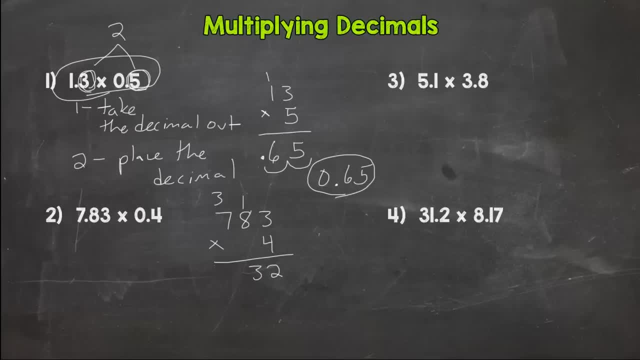 seven times four is 28 plus three is 31, so you get 3132. now go back to your original problem. see how many digits are behind a decimal: one, two, three. so that means our answer will have three digits behind the decimal. So I bring it in three: One, two, three. So our answer is three and 132. 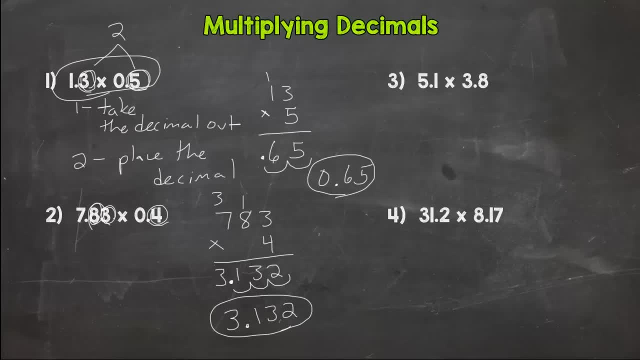 thousandths Boom. Done with that one. So number three: What's our first step? Hopefully you're thinking: take the decimal out. So we do 51 times 38.. Eight times one is eight. Eight times five is 40.. Done with the eight. We need a placeholder zero for this three here. 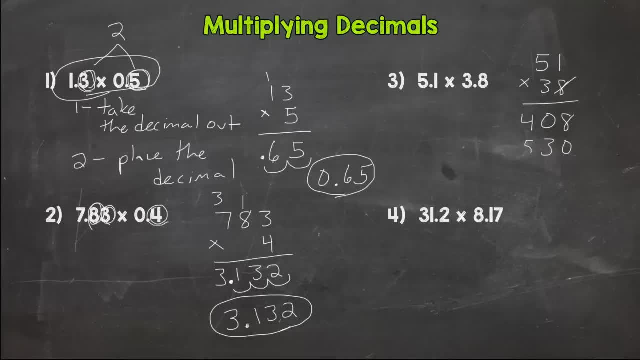 Three times one is three. Three times five is 15.. We need to add our partial products here And we get 1938.. So let's check, take a look and check our original problem. We have one, two decimals or two digits behind, or to the right of a decimal.